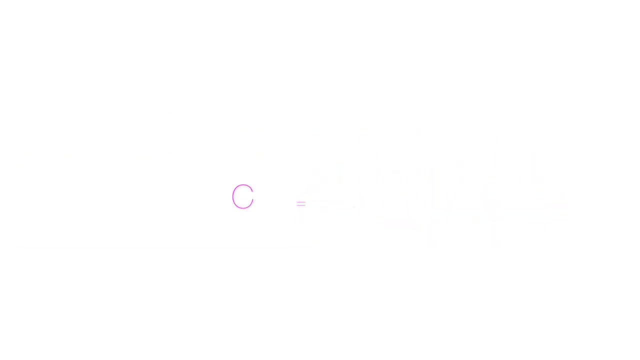 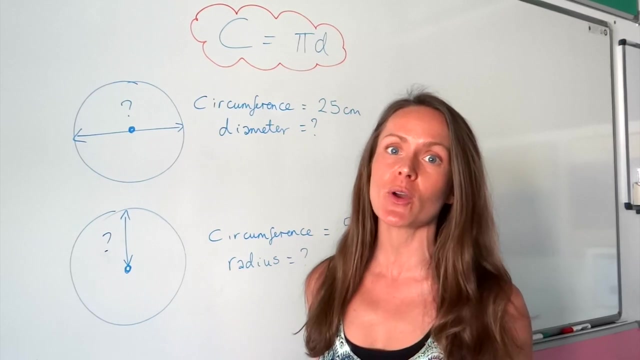 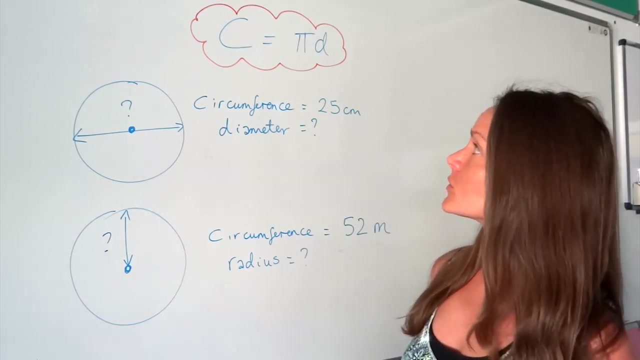 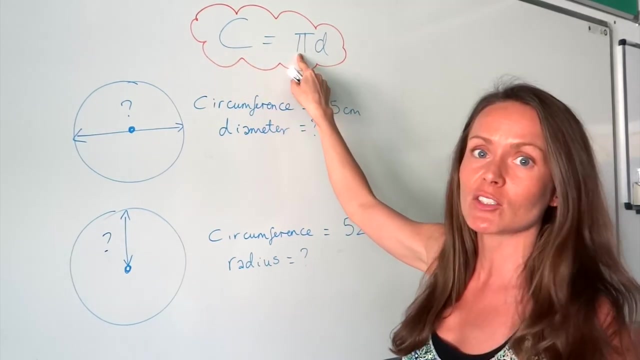 Hey guys, in this next video I'm going to show you how to work out both the diameter and the radius of a circle when you know what the circumference is. So the equation to work out circumference is up here: C equals pi, d. C is just the circumference, Pi is the irrational number, 3.142, and the diameter. 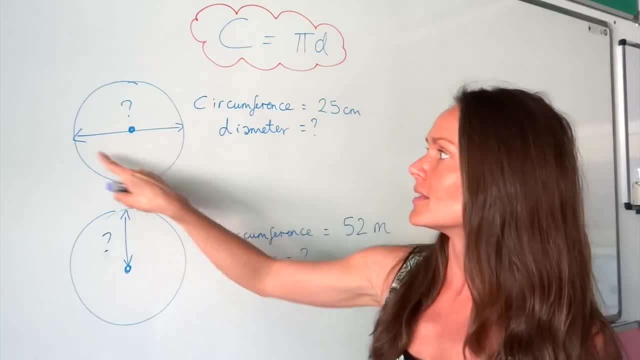 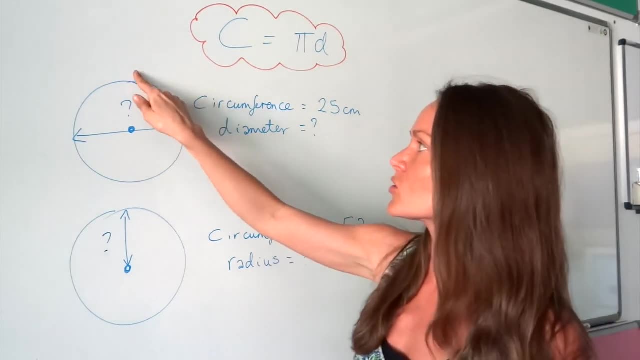 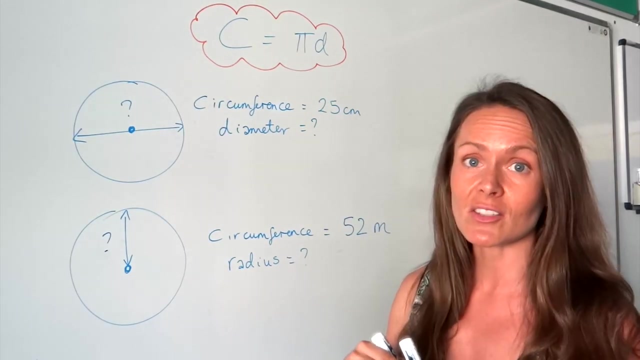 is the distance all the way across the circle, like in this diagram here. Now, remember, circumference is just another word for perimeter when we're talking about circles, So it's just talking about this distance around here. Now, when we have these questions, the best thing to do is to start by. 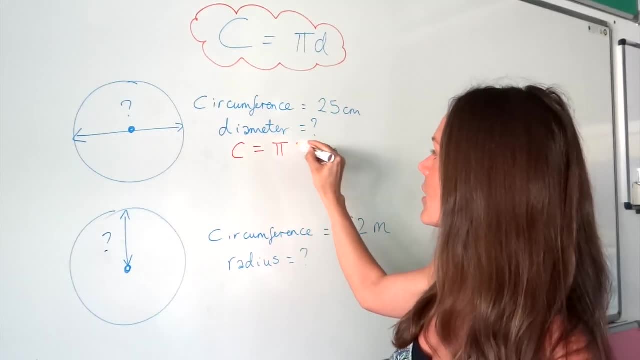 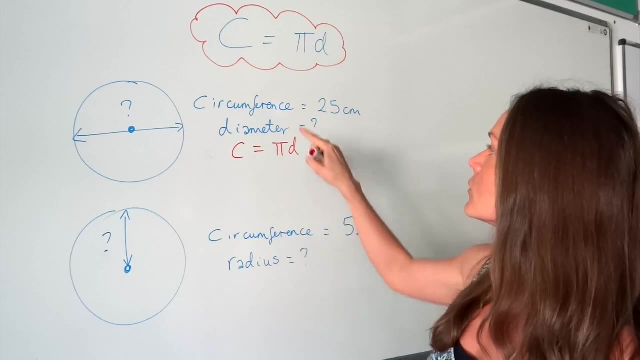 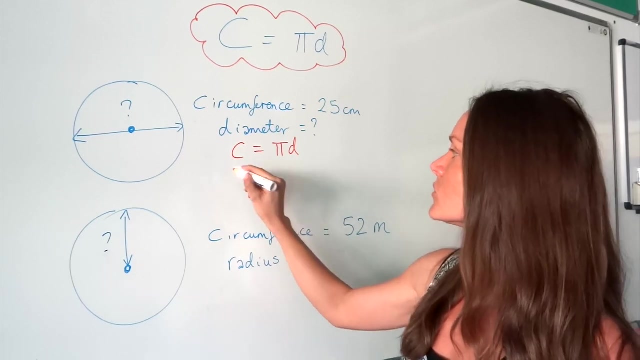 writing down the formula for circumference, So pi d. Then you should substitute in the information that you know: So in the first one we know that the circumference, this distance here, is 25 centimeters. So I'm going to change c, which is the circumference, to 25.. Now, remember, we're trying to 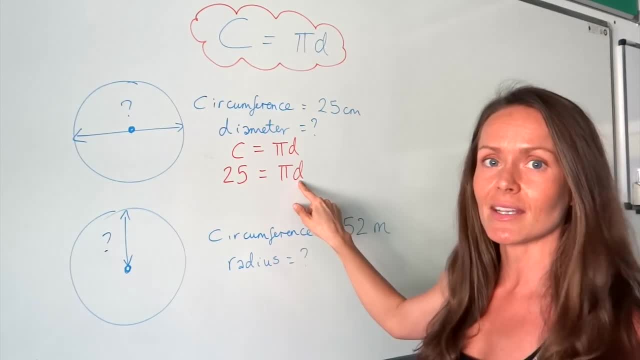 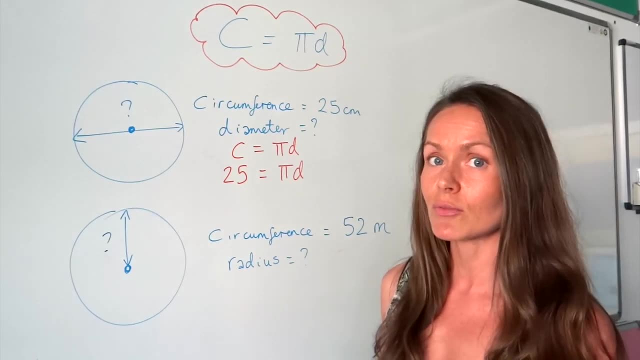 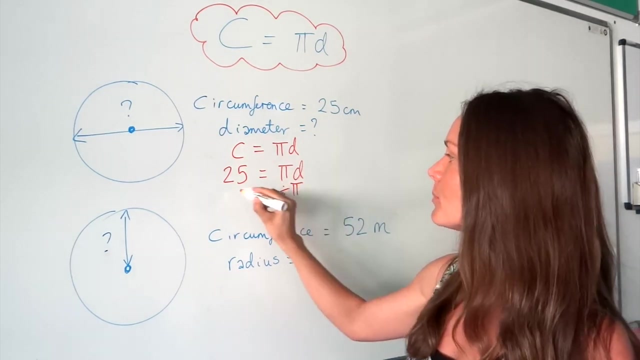 find the diameter, this distance here, which is d in the equation, But d is being multiplied by pi. So what I need to do to solve this equation, to find d, I need to do the opposite And instead of multiplying by pi, I need to divide by pi. Remember, when you're solving equations, you have 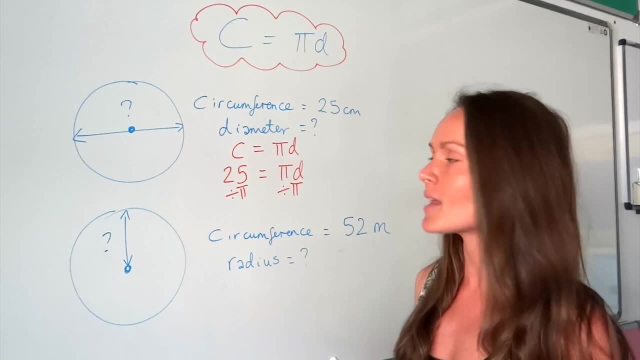 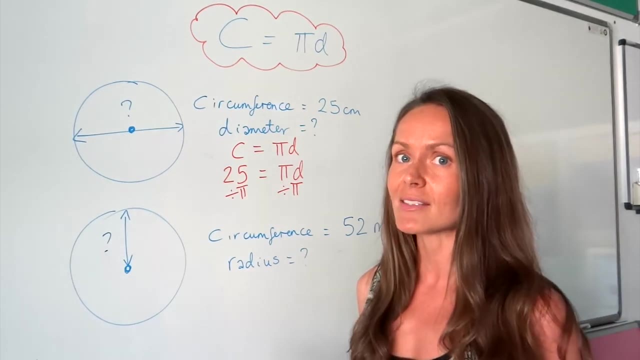 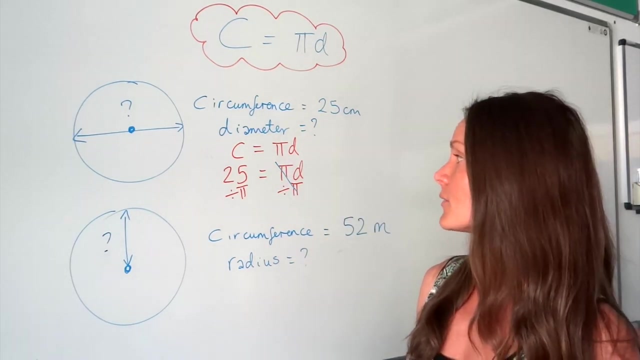 to do the same thing to both sides of the equation to keep it balanced. So on the right hand side, when I do pi divided by pi, remember when you divide something by itself you get 1.. So pi divided by pi leaves you with 1d, And on the left hand side, all that's left to do is to calculate. So 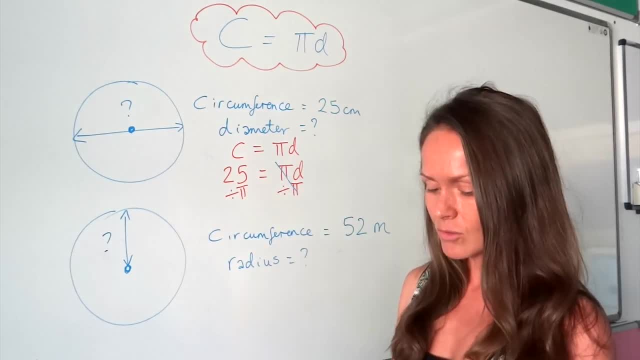 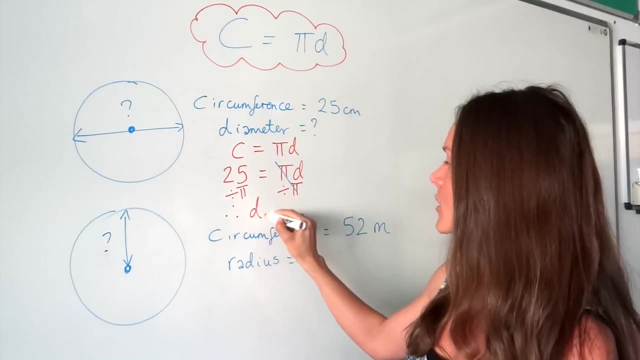 you actually put that part in the calculator and do pi, d divided by pi, And you have to do this, So 25 divided by pi. Now that gives me the answer to D. So D is equal to 7.957. dot, dot, dot. 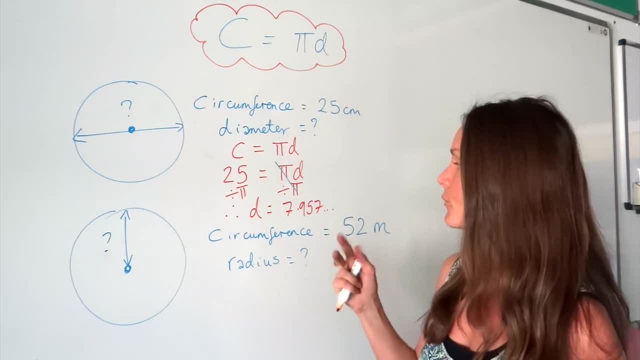 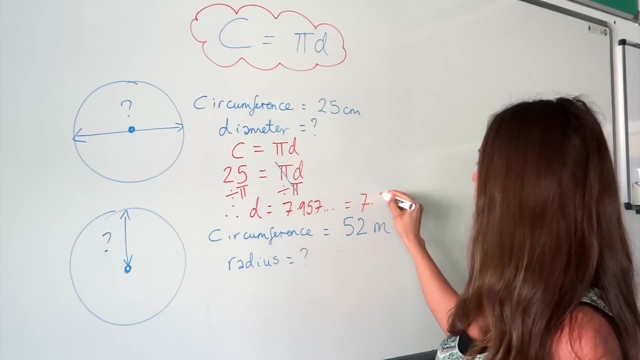 And I'm going to round my answer to three significant figures. So I want three numbers in my answer, So 1, 2, 3.. But that 7 rounds the 5 up to 6.. So it's 7.96.. Remember to include. 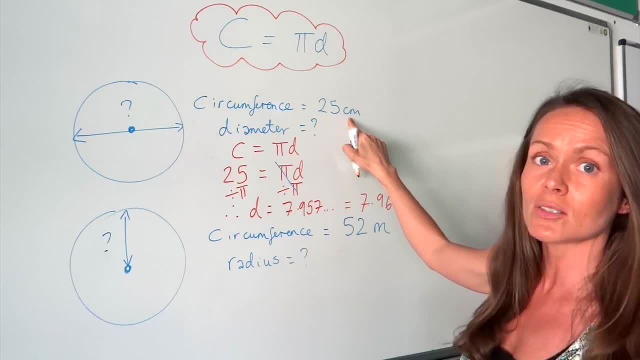 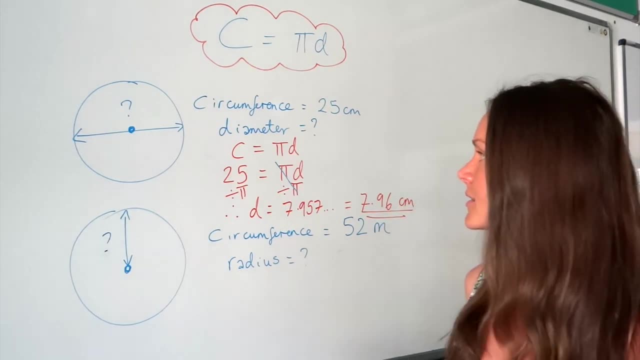 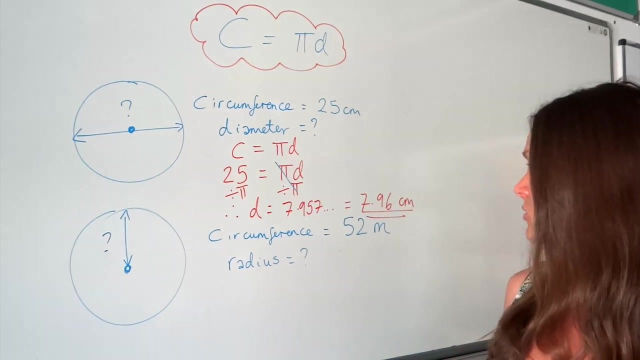 the units. in this question The circumference is given in centimetres, So the diameter is also in centimetres. OK, so that's the first one done. That was really easy. All you had to do was divide the circumference by pi to find the diameter. OK, now on to the next. 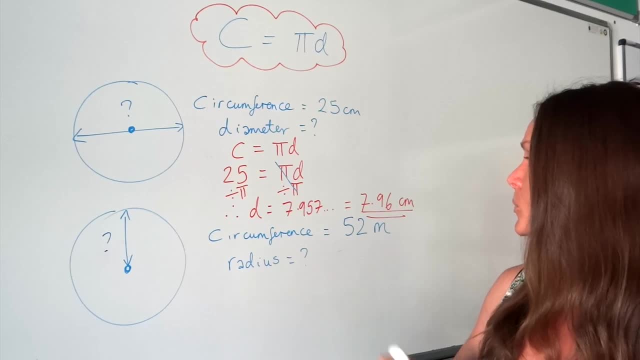 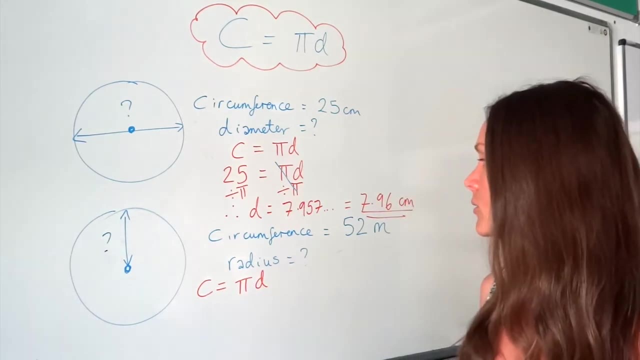 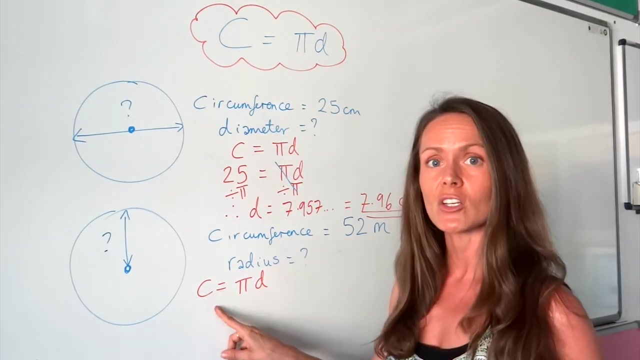 one. So we're going to start the same way And because we're given the circumference, I'm going to write down the formula for circumference. So C equals pi D. Now don't worry That in this question it's asking for the radius And we don't have R in our equation. 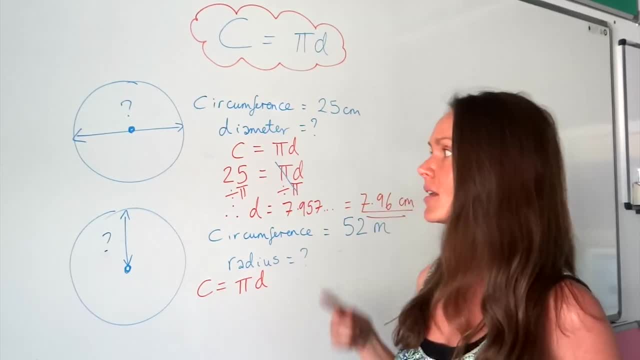 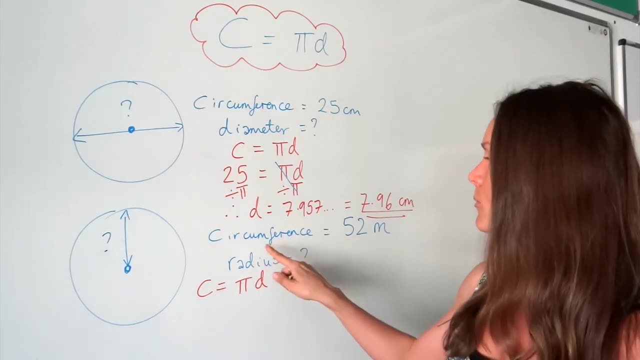 We'll worry about that later. First let's just find the diameter, like we did in the first example. So the next step is to just substitute in what you know. So remember we are given the circumference is 52 metres. OK, so this distance is 52. So I'm going to 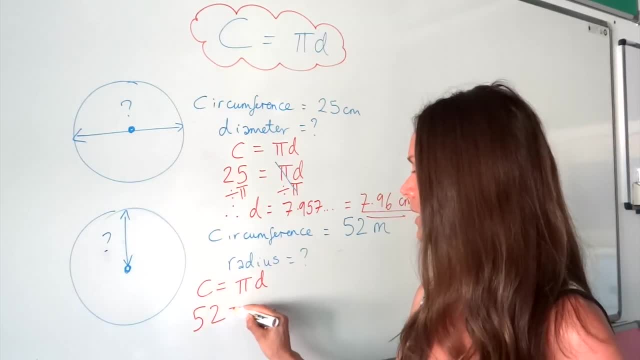 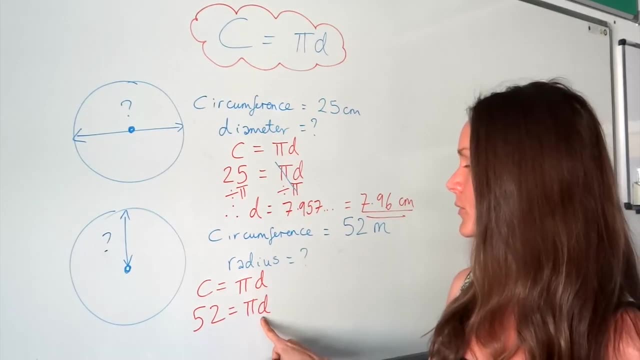 change C to 52. And that leaves me with pi D. Now let's look at the next one. So I'm going to write down: the circumference is 52 metres. Now, just like in the example up here, to find the value of D, the diameter we need. 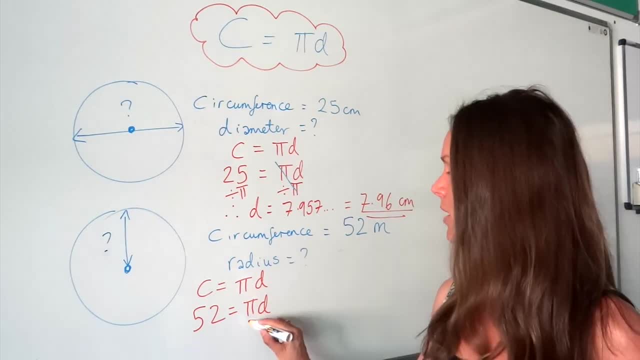 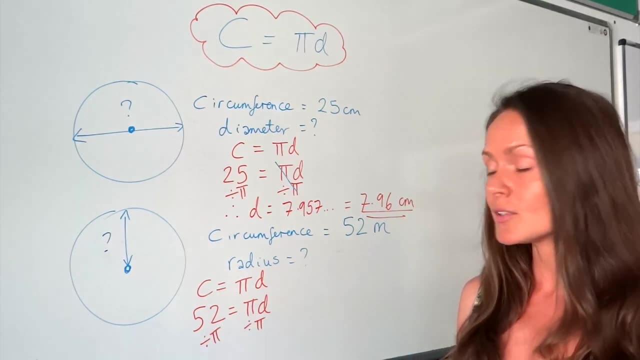 to divide by pi. And remember, if we divide by pi on the right-hand side, we must do the same on the left-hand side. So here, pi divided by pi gives me 1D. I'm just left with 1.. And 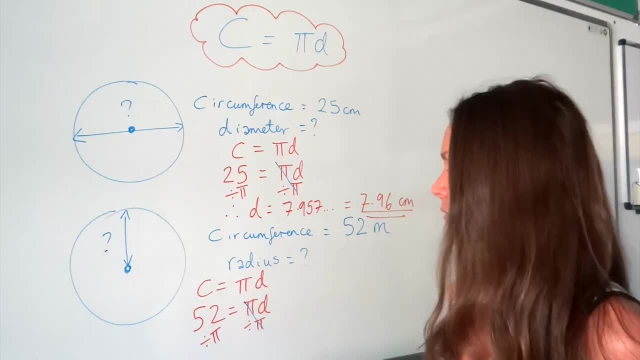 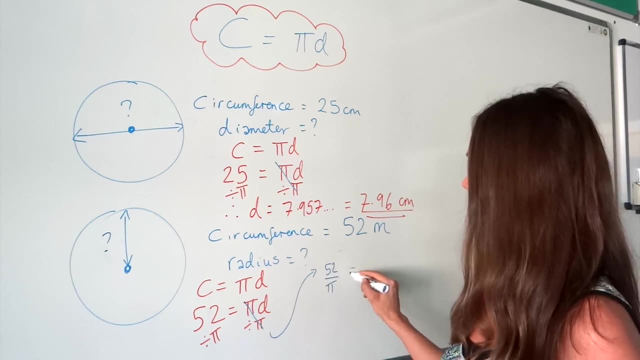 if I do 52 divided by pi, it works out the diameter. So I'm going to write it up here. So 52 divided by pi, It gives me the diameter, And when I put that in the calculator it's probably going. 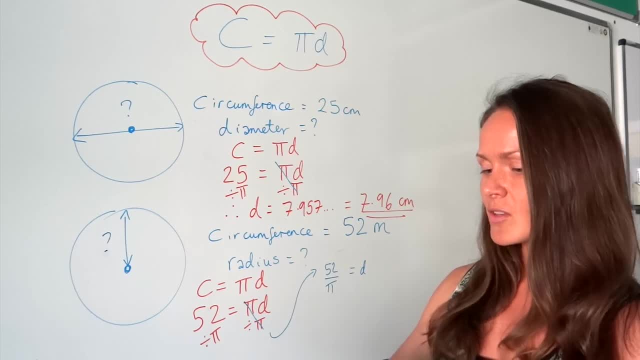 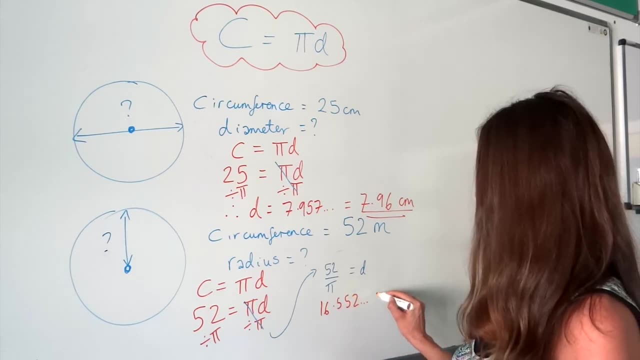 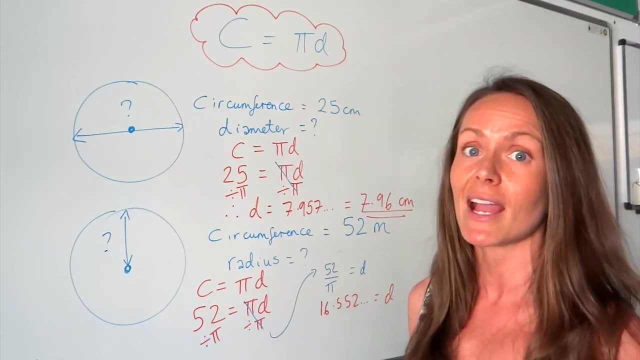 to give me a long number here, lots of decimals, So it gives me 16.552.. So leave that answer on your calculator screen. We don't want to start rounding during the question, because we want our answer at the end to be really accurate. So this is the diameter. Now let's 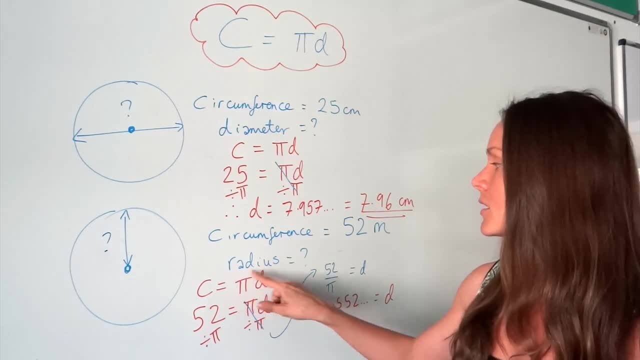 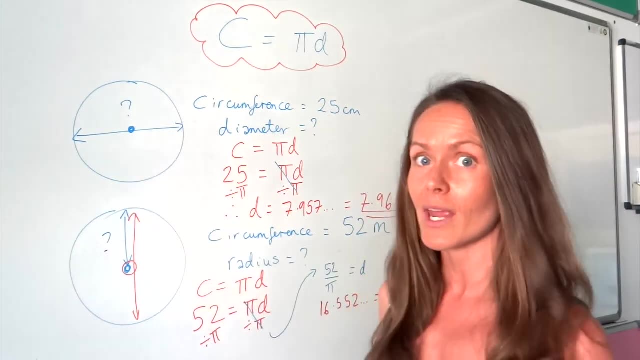 remind ourselves what it's actually asking for in this question. It says: find the radius. Well, we've just worked out the diameter, which is the distance. remember all the way across the shape, So that distance is 16.552.. But we only want: